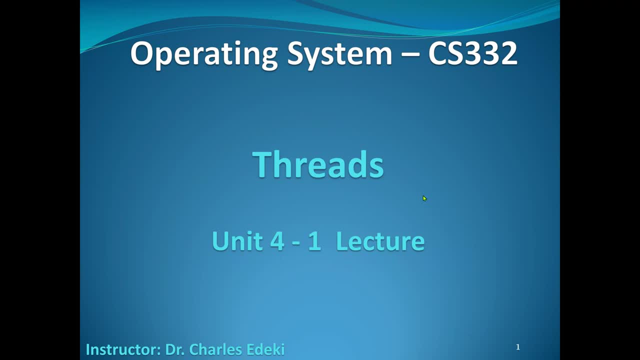 or a program that is executing. So a thread also is a program that is executing. but a thread will be a mini process, which means again, one process can have two or more threads. So all the characteristics of a process is almost the same as a thread. So the discussion so far has presented: 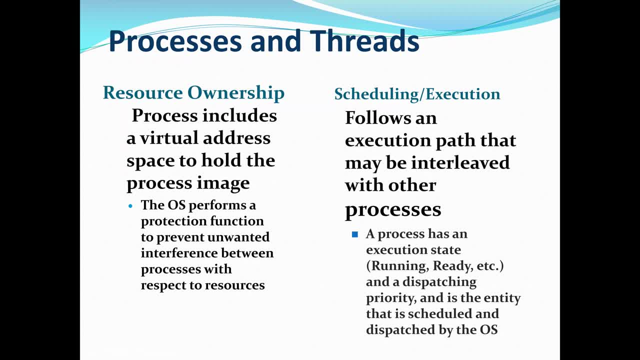 the concept of a process as embodying two characteristics, that is, resources ownership and also schedule and execution. So a process includes the eventual address space to hold the image or the process image, If we can record this. in chapter three of our course textbook we said the process image is the collection of program. 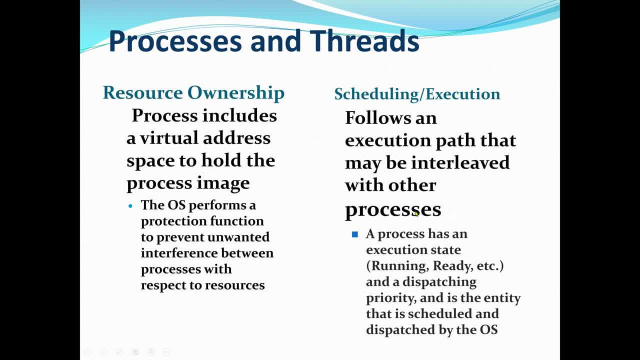 stack data and attributes that define in the process control block. So from time to time a process may be allocated control or ownership of resources. First of all, a process requires, for example, context of some number of raw materials or any scenery Or system Or the kernel of the node. 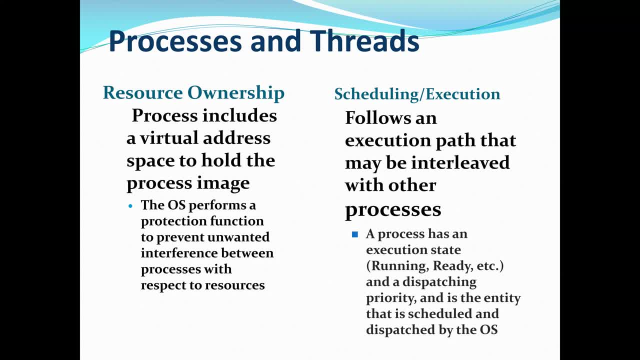 of the node, of the node. Finally, the process: boundary development of links's activity structure. To do this, Once you discuss of a process- and the topic is one of the major obstacles- past and present aspects of the processes. both are related to landscape optimization And so you can review. So, first of all, what is the biblical approach to regulation? It's basically a process. The ruler of this is the pillar which 고양me attention toif a good. So, first of all, what are conceptual concepts in the development of an, an application? 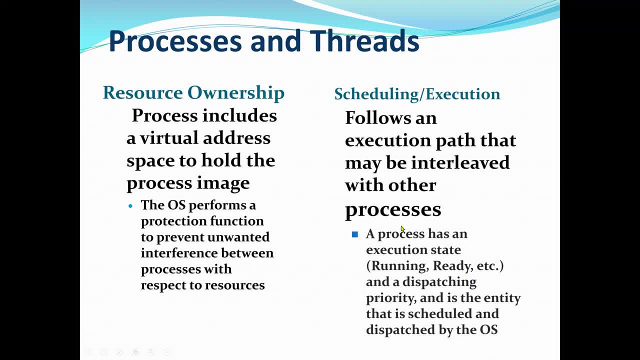 So students should consider that they are typical, would say institutional, well considered for top ». assume a action that involves Aha la and the lateral ethic, such as classical, environmental. how are they effect and not theoretical outcomes? in nearly one or a few other games Now with a scheduled execution, normally we know that as the execution of a process follows, 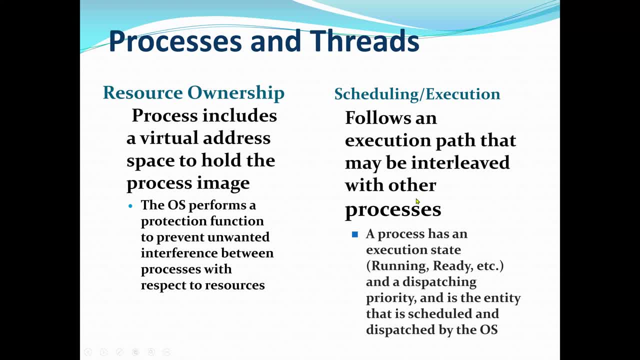 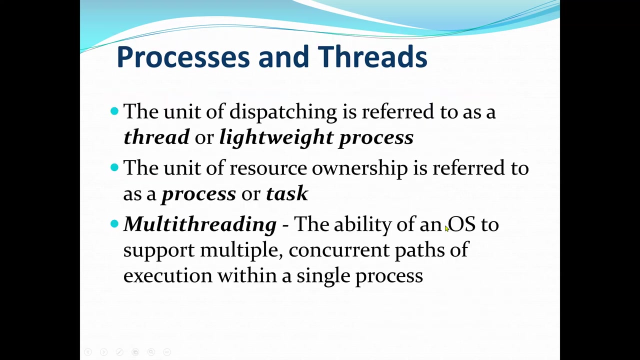 an execution path which is the trace through one or more programs, So this execution may be interleaved with that of other processes. So we can see a process has an execution state, such as running or ready, and also a dispatching priority and is the entity that is scheduled and dispatched by the operating system. 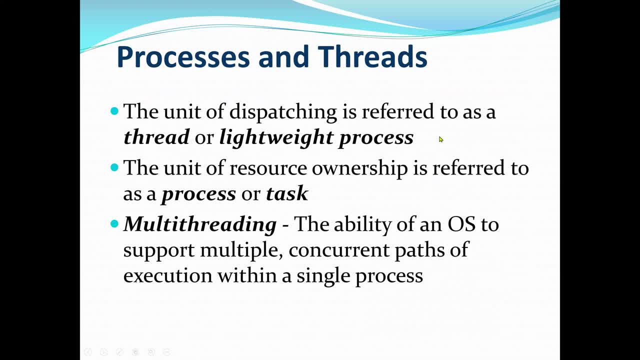 Now the unit of dispatching is referred to as the thread or lightweight process. So, as we said again, process and thread have almost the same characteristics, the same function, everything. So a process, or we say a thread, is a lightweight process, which means again, a process can. 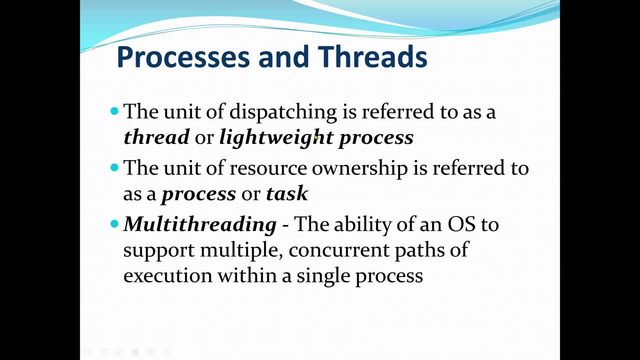 have many threads, So some unit of resources ownership is referred to as a process or a task, And also multi-threading means the ability of an operating system to support multiple concurrent paths of execution within a single process, So which means we have a single process. 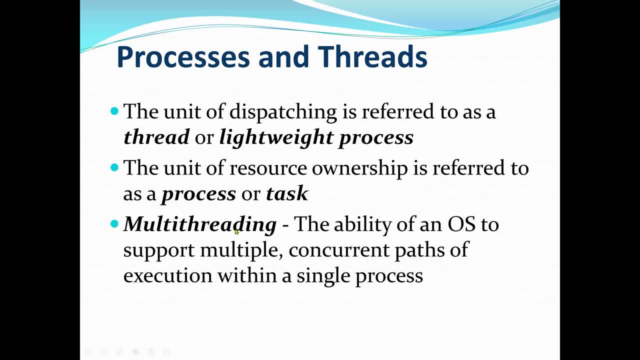 That is executing, but it may have multi-threading, which means it can have two or more threads. Each thread will be a task which normally will be executed concurrently. So some thought should convince us that these two characteristics are again independent and could be treated independently by the operating system. 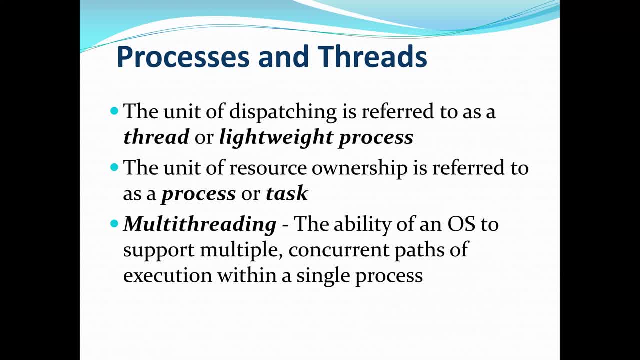 And this is done in a number of operating systems. So let's look at some of the characteristics of multi-threading and multi-threading as well. Now, to distinguish the two characteristics, the unit of dispatching is usually referred to as the lightweight process, while the unit of resources ownership- is referred to. 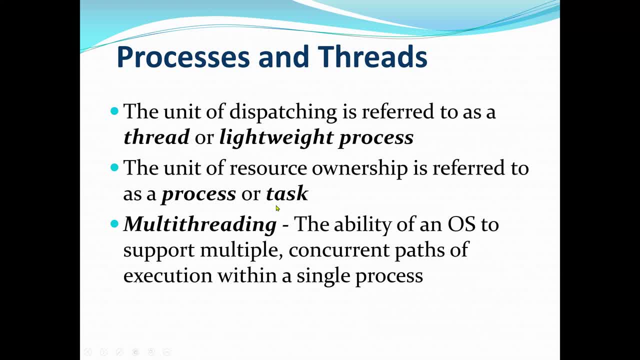 as the process or the task. So again, multi-threading refers to the ability of an operating system to support multiple concurrent paths of execution. Now, to distinguish the two characteristics of multi-threading and multi-threading, let's look at some of the characteristics of multi-threading and multi-threading. 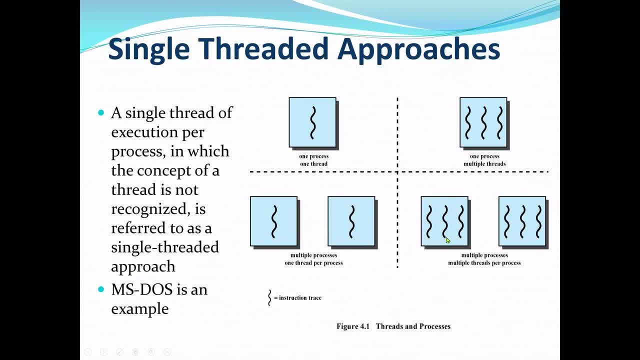 The unit of dispatching refers to the ability of an operating system to support multiple concurrent paths of execution within a single process. So here we have a very good example, a traditional approach of a single thread of execution per process here, in which the concept of a thread is not recognized. 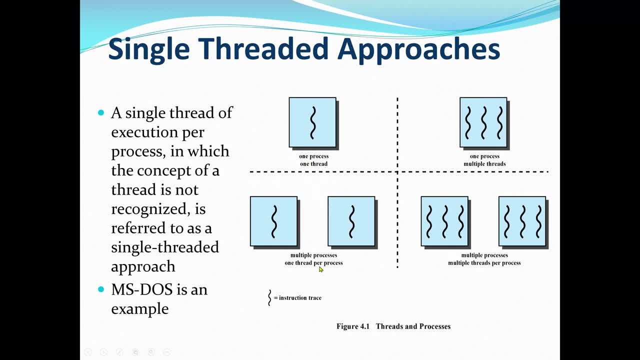 So here we have one process, one thread And this section we have multiple process, That is one thread per process, But we may also have one process with multiple threads. So here we have one process with three threads, Or we may have a multiple process with multiple threads. 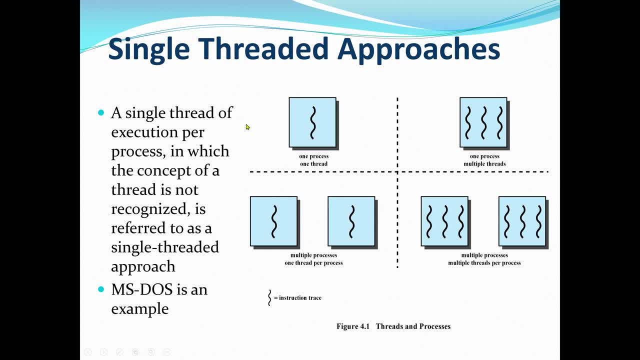 So again, the traditional approach of a single thread of execution per process, in which the concept of thread is not recognized. This is referred to as a single thread approach. So on our left side, again we have a single thread approach. Now two arrangements show: 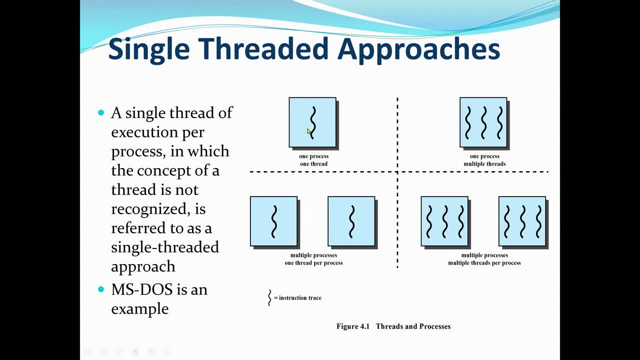 In the left half of this, our figure 4.1, a single-threaded approach. So Microsoft does or MS does. it's an example of, again, an operating system that supports single user process and single thread. Now on our right side, again, we have the multiple thread. 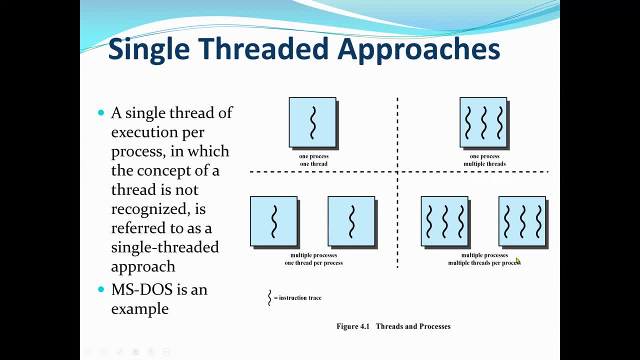 We can have a single process, multiple thread Or multiple process. So other operating systems, such as Unis, support multiple user process but only support one thread per process, And the figure here again shows multi-threading threaded approaches. 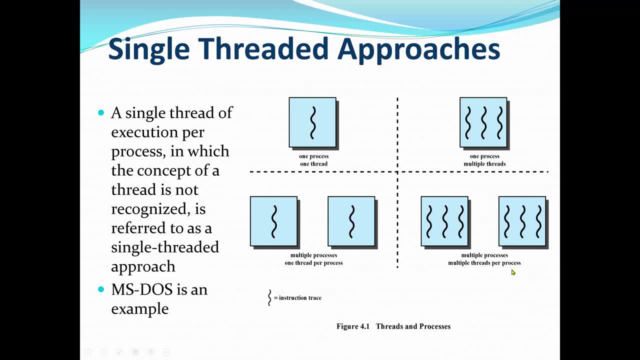 So a Java runtime environment is an example of a system of one process with multiple thread. So this is an example of a system of one process with multiple thread, And the figure here again shows multi-threading threaded approaches. And the figure here again shows multiple user process approaches. 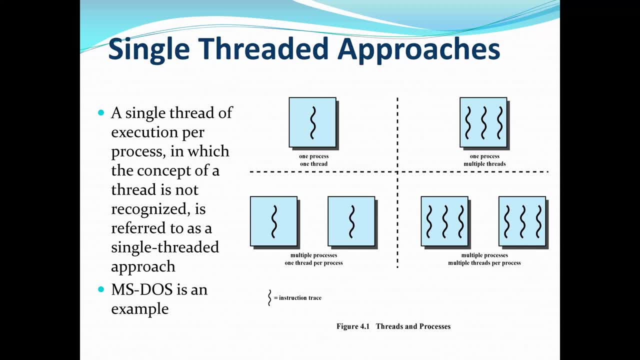 And the figure here again shows unicubal analysis. So this is an example of a system of one process in which one user can have multiple threads. Also of interest is the section the use of multiple processes, of which support multiple threads. 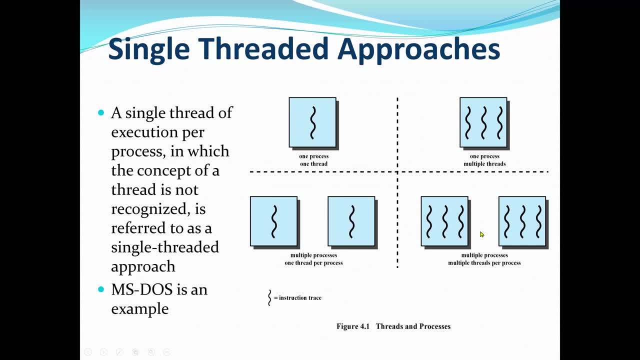 And this approach again is used in Windows, Some many modern versions of Unis and Linux operating system. So in this session we will give a general description of multi-threading and also the details of Windows, Solaris and Linux. 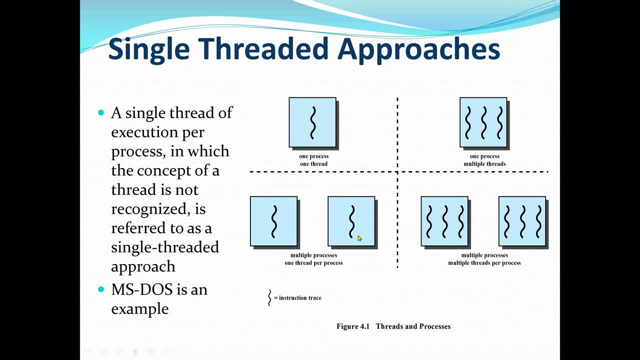 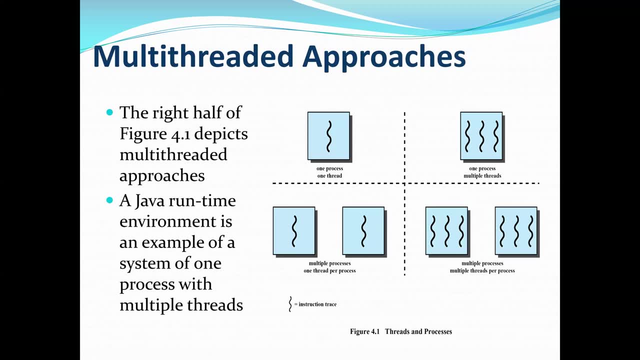 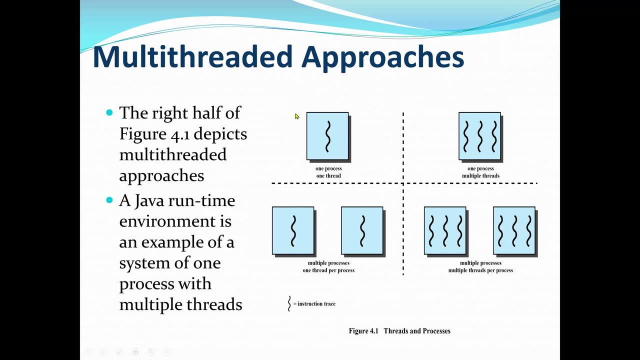 Next slide. blindness approach will be discussed later in this chapter of our course textbook. So again, in a multi-threading environment, a process is defined as the unit of resource allocation and also a unit of protection. So again, the following are associated with process. 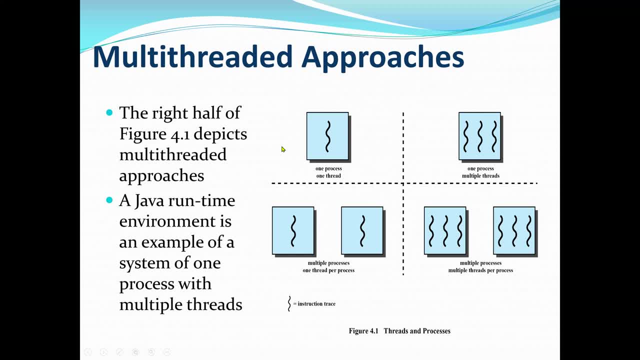 the venture address space that holds the process image, and also the protected access to processes or other processes, Also the inter-process communication files, the IO resources such as the channels and the device. So from here we say the right half of the figure 4.1. 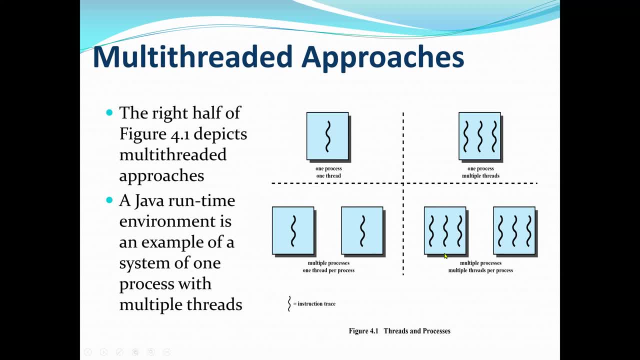 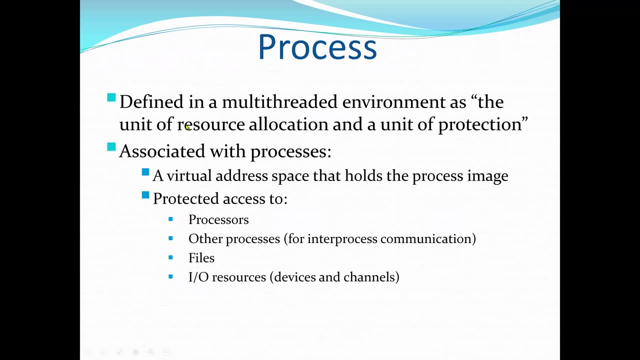 shows the multi-threading approaches also And Java Runtime Environment is an example of a system of process and one process with multiple threads. So process is defined, as we said again, in a multi-threading environment as a unit of resources allocation and also unit of protection. 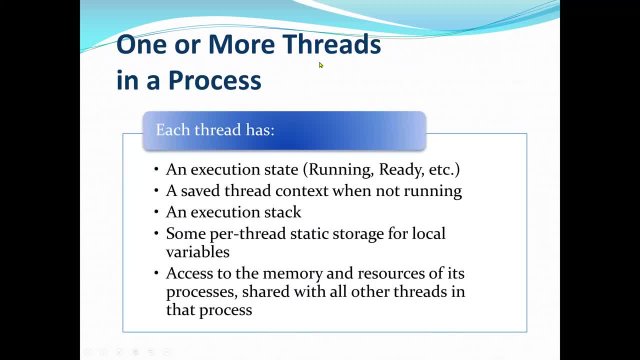 So we have one or more of these processes. So we have one or more of these processes. So we have one or more of these processes, One or more threads in a process. So again, we need a process that may be one or more threads. 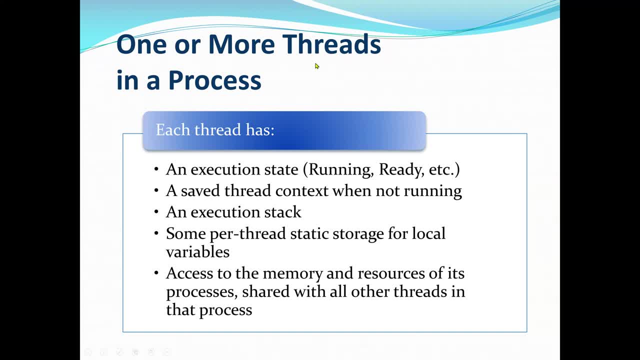 Each with the following: Every process, one or more thread. At least we may have a thread execution state which can be running already and also a safe thread contest when not running. One way to view a thread is an example. One way to view a thread is an example. 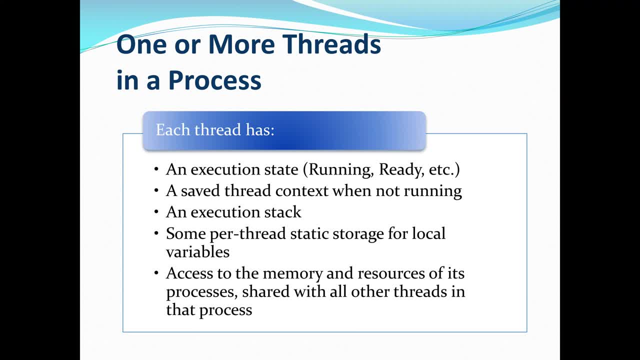 an independent program counter operating within a process. Also we may have the execution stack or some pair thread stack storage for local variables. Again some pair thread strategic storage for local variable. Also access to memory and resources of its process share with all other threads in that process. 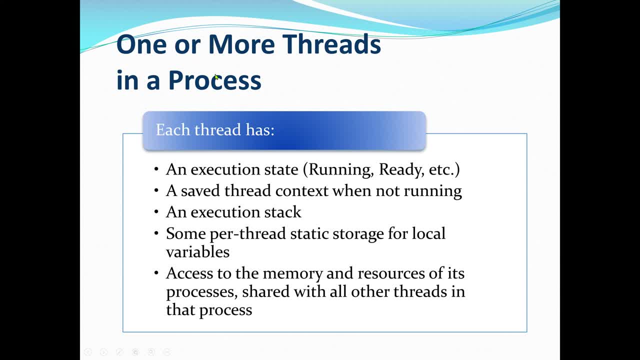 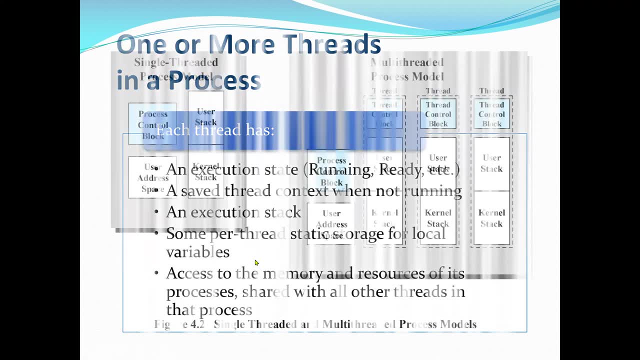 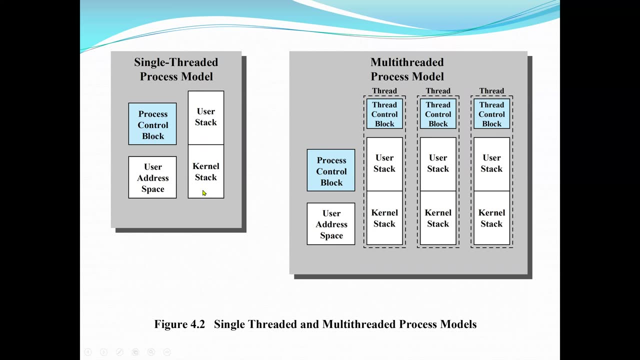 So again, one or more threads in one process or in a process. Now each thread may have all these characteristics. So that's example here in this figure here shows the distinction between thread and process from the point of view process management. So we have single thread process model. 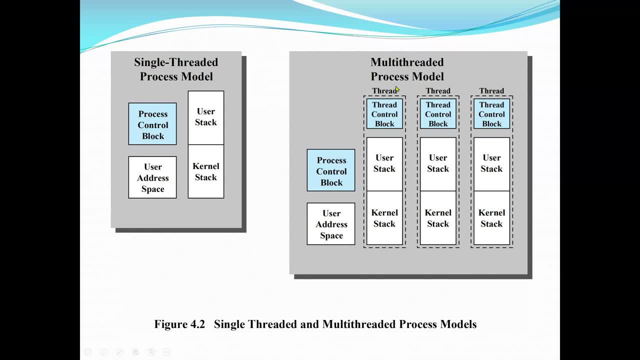 multi-threaded process model. So we can see in one system we have different threads, each is a thread And we may have the thread control block with the user stack and the kernel stack, Also the process control block and the user thread space. 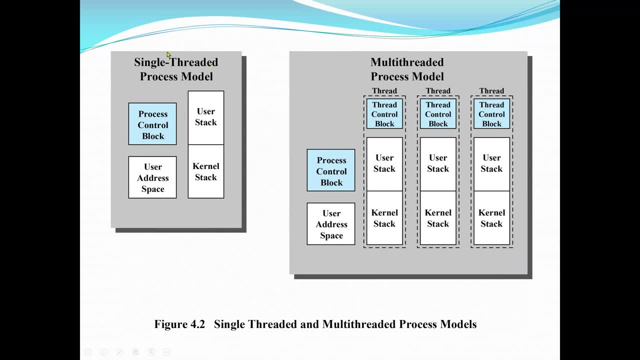 And this is a single threaded process model. So in this case we have only one thread. In our right we have multiple threads. So the representation of a process include is process control block And also the user address space as well as other user and kernel stacks. 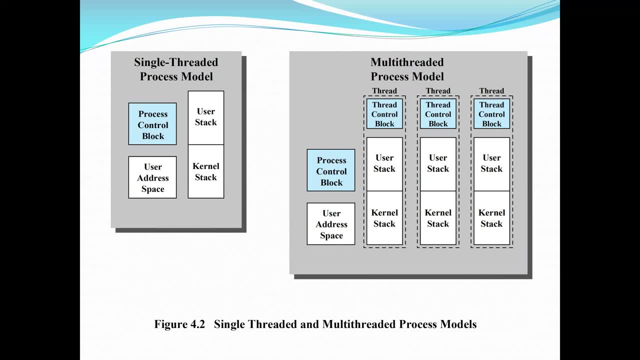 to manage the call return behavior of the execution of the process. Now, while the process is running, it controls the processor registers And the content of these registers are saved. when the process is not running, Now, in the multi-threaded environment there's still a single process control block. 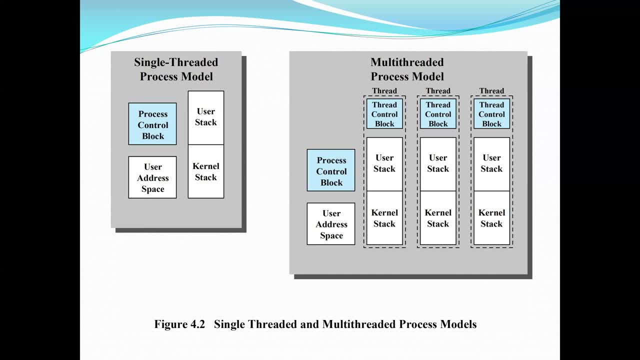 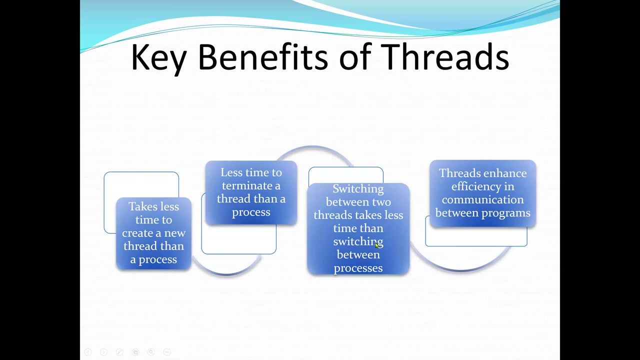 and also a user screen address space associated with this process. but now there are separate stacks for each thread. as we can see in the diagram, we have a single process control block user address, but each thread have its own user stack, kernel stack. so the key benefit of threads: here we say, based on this concept, all of the threads of a process. 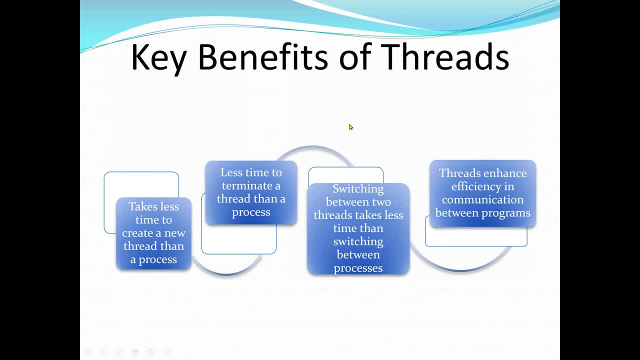 will share the state and also the resources of that process. so we have one process. it may have 10 different threads. all the threads must share the same state and the resources of that process and this is the key benefit of this process. so we say, based on this concept, all of the threads. 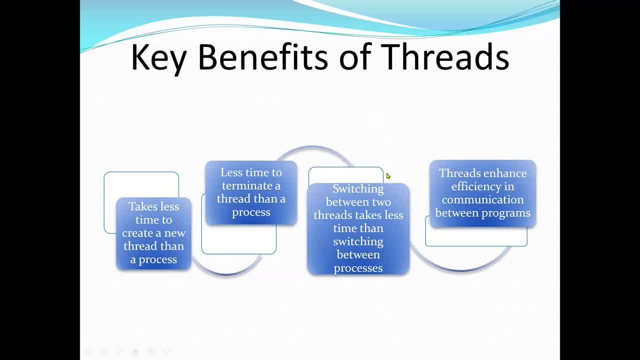 may reside in the same address space and also have access to the same data. all the thread may have access to the same data because they all belongs to the same process. now, when one thread utters an item of data in memory, then the other threads see the result- if, if and when they access. 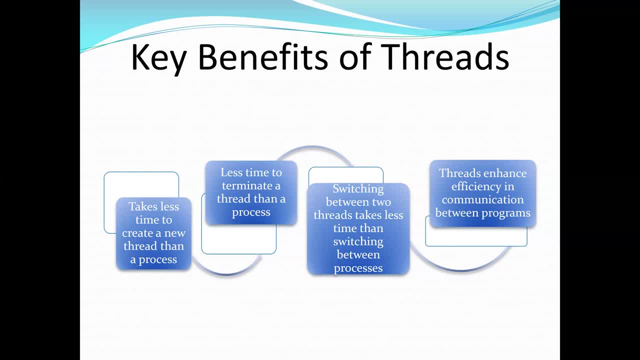 that item. so again, if one thread opens a file with read privilege, other threads in the same process can also read from that file. now the key benefit of thread derived from the performance implications. so one is: it takes far less time to create a new thread in an existing process than to create. 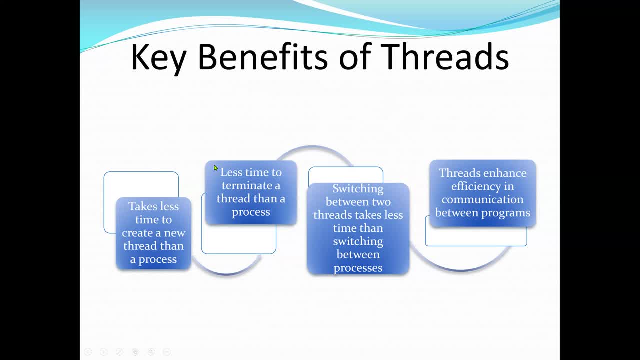 a brand new process and also studies- it was done by max developers- which shows that a thread creates another thread, that the thread creation is 10 times faster than the process creation in UNIS. Also the second benefit: it takes less time to terminate a thread than a process. 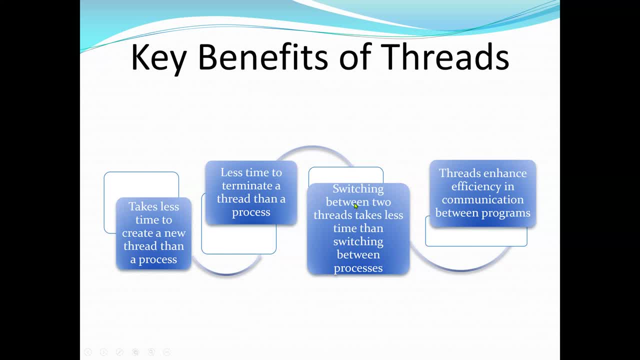 And third also, it takes less time to switch between two threads within the same process than to switch between processes. And lastly, the thread enhance efficiency in communication between different executing programs. So in most operating system communication between independent process requires the intervention of the kernel. 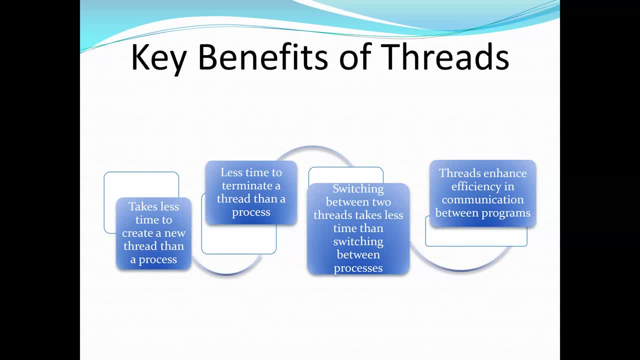 to provide protection and mechanism needed for the communication. However, because threads reside within the same process and they share the same memory and files, they can communicate with each other without invoking the kernel. So here we can see if there's an application or a function that should be implemented. 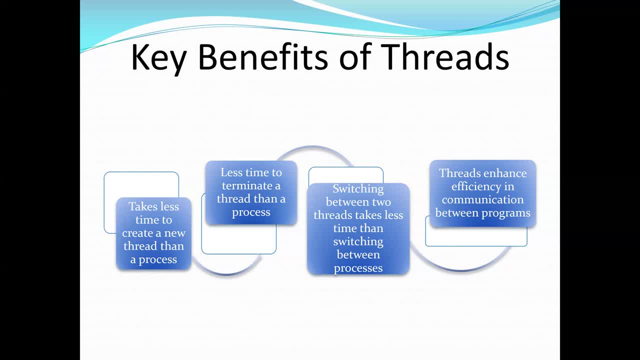 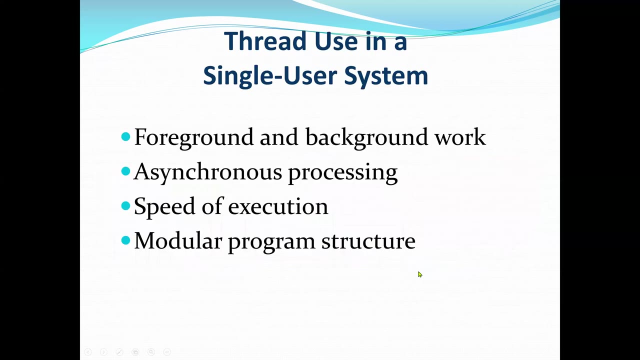 as a set of related units of execution. it is far more efficient to do so as a collection of threads rather than a collection of separate process. So that will be again the main key benefits of thread And so thread use in a single user system. 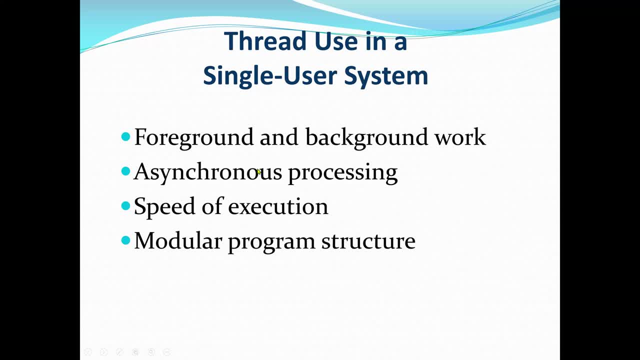 Here we say that there are four different again examples of the use of threads in a single user multiprocessing system. So the first would be the foreground and background work. So for example, in a spreadsheet program one thread should display the menus and read the user input. 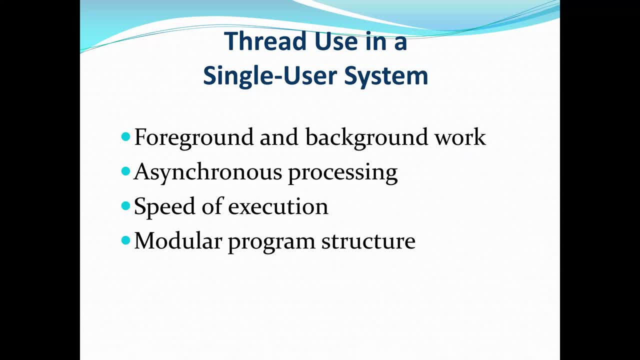 while another thread will execute user command and update the spreadsheets. This arrangement often increase the perceived speed of the application by allowing the program to prompt for the next command before the previous command is complete. And second is asynchronous processing, So asynchronous elements in a program. 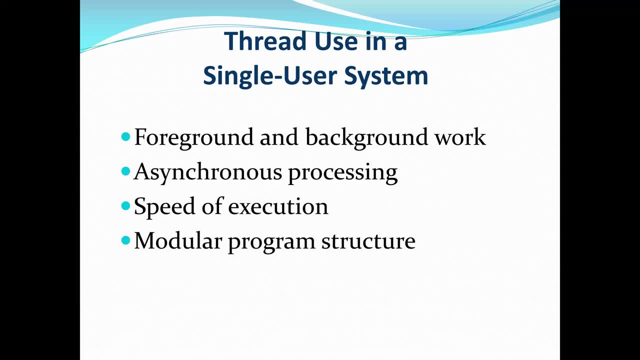 can be implemented as threads, For example as a protection against power failure. one can design a word processor to write its random access memory buffer to Dix once every minute. So a thread can be created whose sole job is periodic backup, and that schedule is set directly again with the. 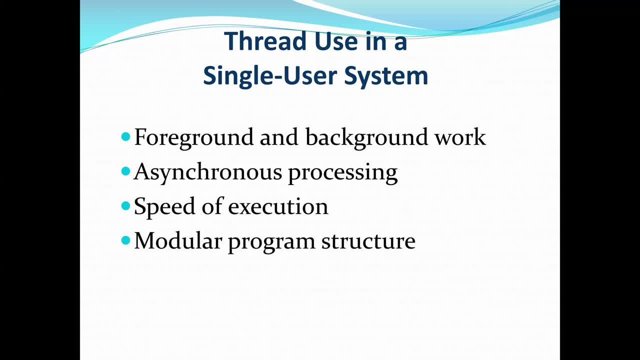 with the operating system. So there's no need for a fancy code in the main program to provide for time checks or to coordinate input and output. Also, the speed of execution is good. A multi-threading process again can compute one batch of a data while reading the next batch from a device. 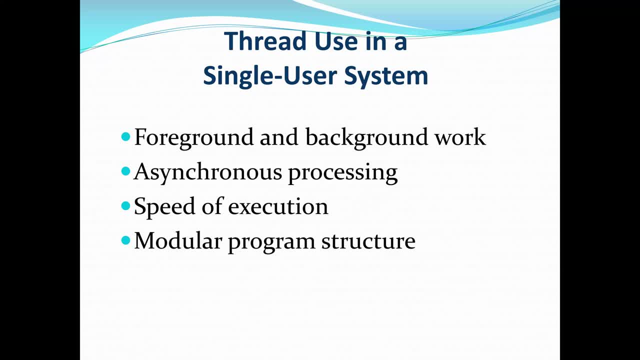 So on a multiprocessor system, multiple threads from the same process may be able to execute simultaneously. So even though one thread may be blocked for an input and output operation to read in a batch of data, another thread may be executing, And also the modular programming structure. 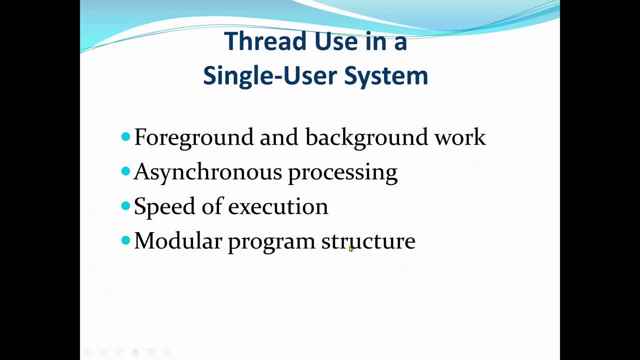 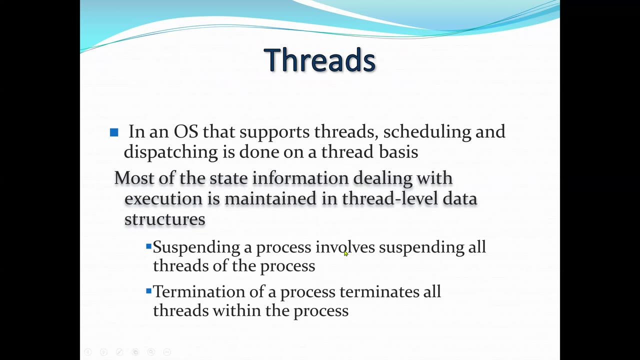 So programs again, that invoke a variety of activities or a variety of resources and destination of input and output, may be easier to design and implement Using again threads. So again in an operating system, operating system that support thread, scheduling and dispatch is done on thread basis. 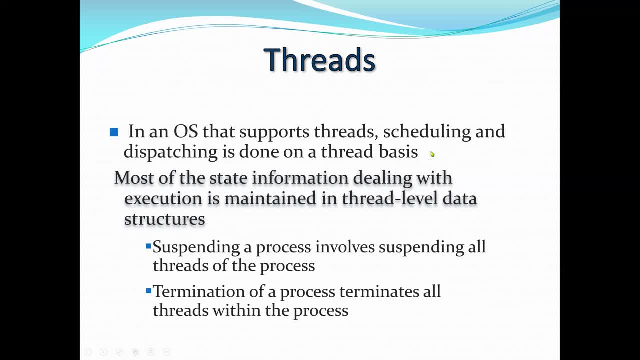 Again because of the efficiency and the speed also. So most of the state information dealing with execution is maintained in the thread level data structures, But also there are several actions that affect all of the threads in a process and that the operating system must manage at the process level. 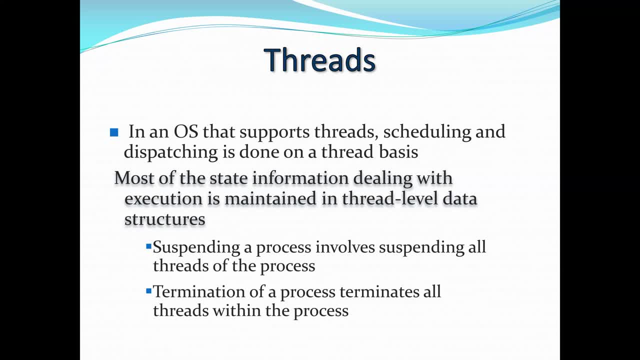 So, for example, example, suspension involves swapping the address space of one process out of main memory to make room for the address space of another process. And because our threads in a process share the same address space, all threads are suspended at the same time. 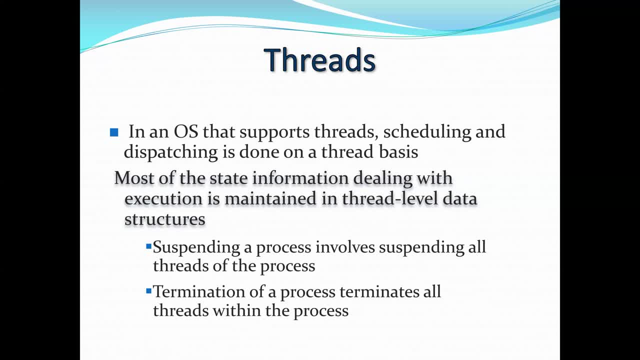 Also: termination of a process: terminate all the threads within that process. So if we have four or five threads in one process, when the process is terminated again all the threads within the process also will be terminated. So thread execution states and the key states for thread again. 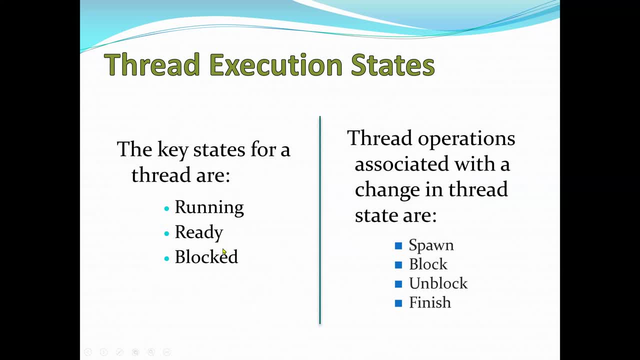 the running ready and also block, And also we may have thread operations that are associated with change in thread states, such as the spawn, block, unblock and also finish. So typically when a new process is spawned, a thread for that process is also spawned. 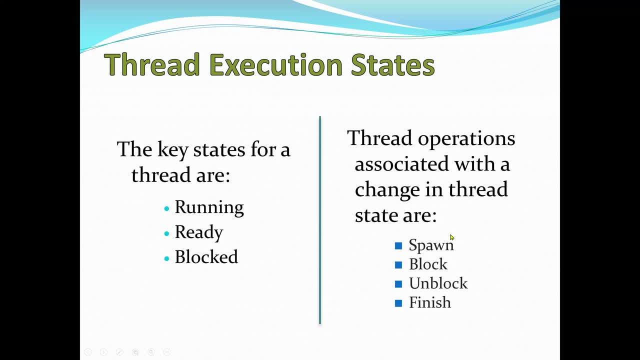 Subsequently, a thread within a process may spawn also another thread within the same process, So providing an instruction, pointer and argument for a new thread. The new thread is provided with its own register, context and a stack space and placed on the ready queue. 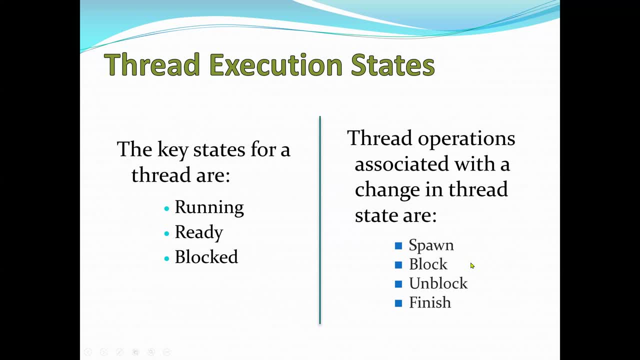 When it comes to blocking or block. when a thread needs to wait for an event, it will block or save its event, And when a thread is moved to the ready queue and is unblocked, its register context and stacks are dead located And this will be the end of the process. 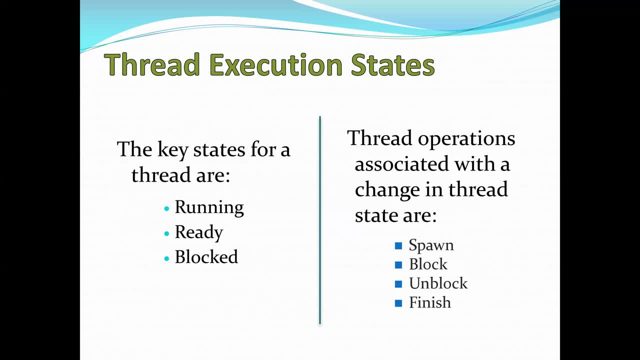 So the process may now turn to the execution of another ready thread in the same or a different process. Unblock is when the event for which a thread is blocked occurs, The thread is moved to the ready queue and is unblocked. And when a thread completes. 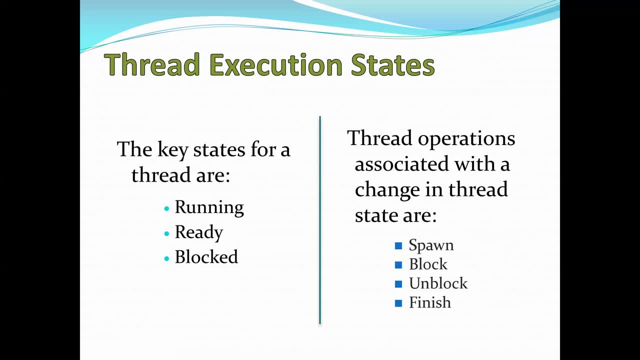 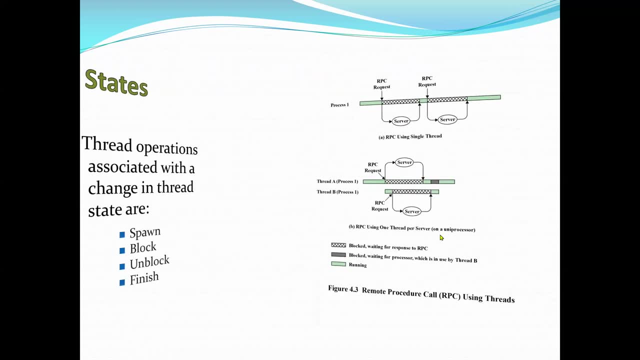 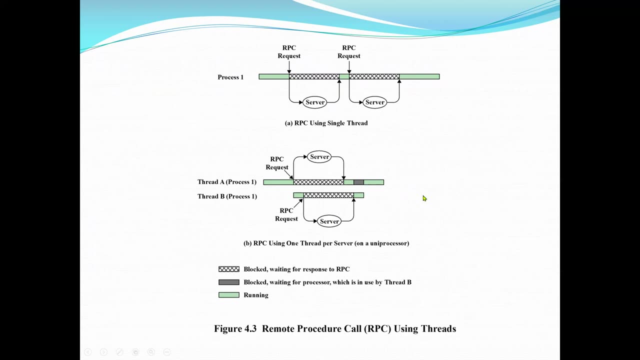 its register context and stacks are dead located And this will be the end of the process And this will lead us to the finish state. So this is an example we have here. So, again, the significant issue is whether the blocking of a thread results in a blocking of entire process. 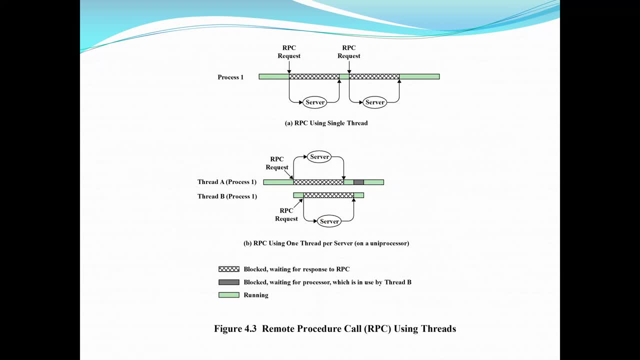 In other words, again, if one thread in a process is blocked, does this prevent the running of any other thread? in the same way, Does this prevent the running of any other thread in the same process, even if that other thread is in ready state? 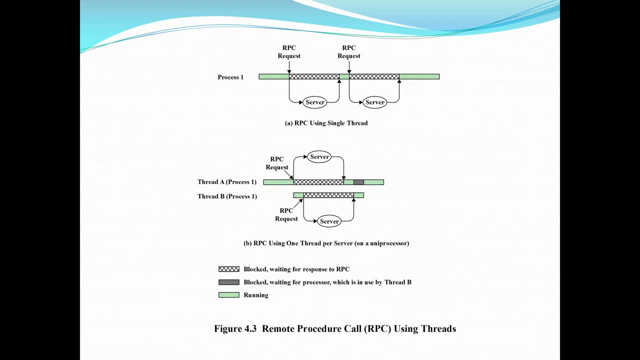 So some of the flexibility and the power of thread is lost. if one blocked thread blocks an entire process. So again, when returning to this issue subsequently, our discussion of a user level versus the connect level threads, but for now let us again consider the performance benefits of threads. 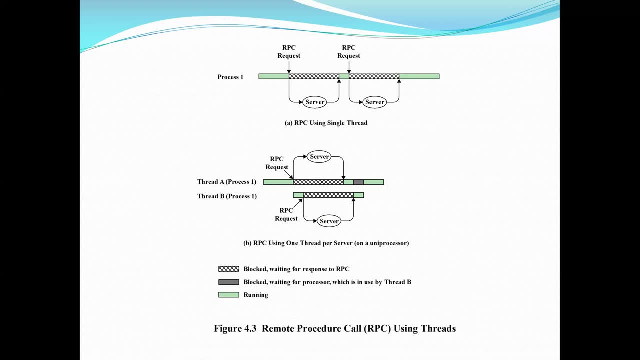 that do not block an entire process. So we can see again. the diagram here shows a program that performs two remote procedure call. So we have the remote procedure RPC requests for two service, two remote procedure calls to two different hosts to obtain a combined result. 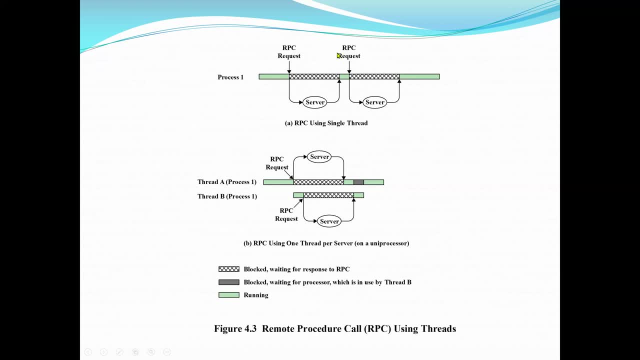 So in a single threaded program the results are obtained in sequence, So the program has to wait for the response from each server in turn. But we can rewrite the program to use a separate thread for each remote procedure. call result in a substantial speed up. 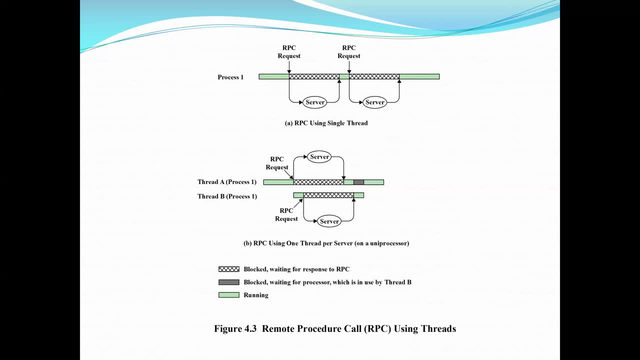 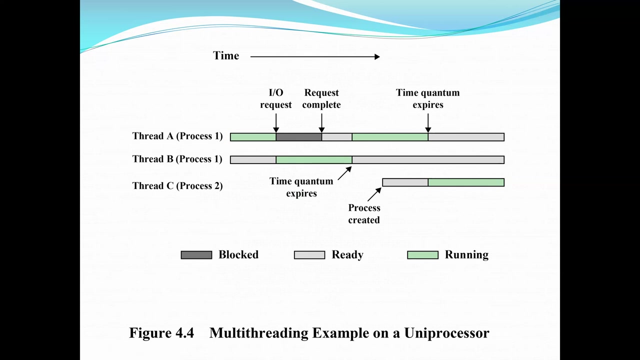 Now, if this program operates on a uniprocessor, the requests may be generated sequentially and the results process in sequence. However, the program waits concurrently for the two replies. So again a one-unit processor. multi-programming enable the interleaving of multiple threads within the multiple processes. 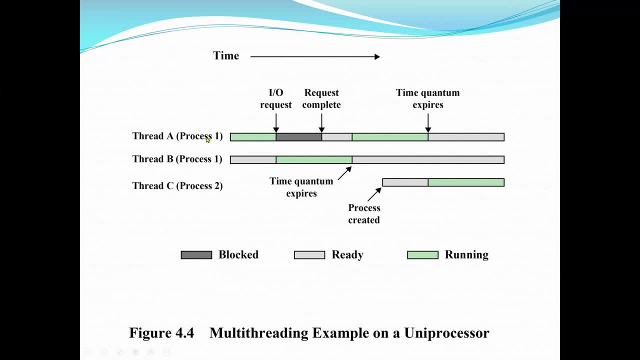 So in this example we have, for example, three threads: A, B and C Process, one, two And three in a two process, three process, three thread in two process interleave on the processor. So here's the cushion: passes from one thread to another, either when the currently running. 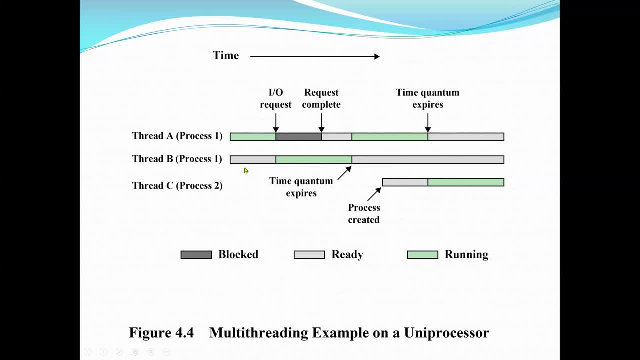 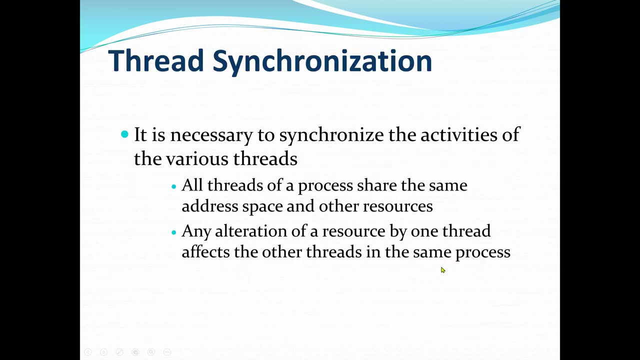 thread is blocked or when it is time, time slice is exhausted. So this is a blocking stage, ready stage and also the running Now with thread synchronization. here we see all of the thread of a process share the same address space. As we said earlier, all threads of one process may share the same address space and other. 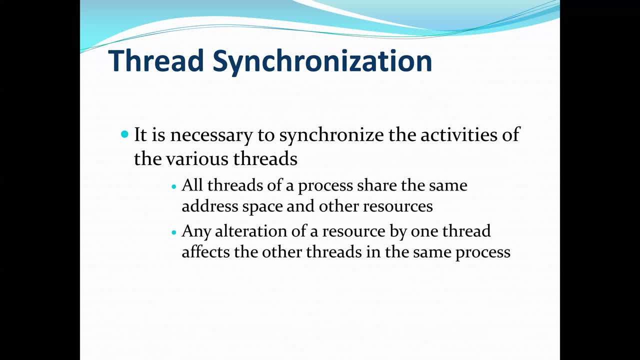 resources, such as again open files or main memory. So any alteration of a resource by one thread will affect the environment of the other threads in the same process. So it's therefore necessary to synchronize the activities of the various threads so that they do not interfere with each other or corrupt the data structure. 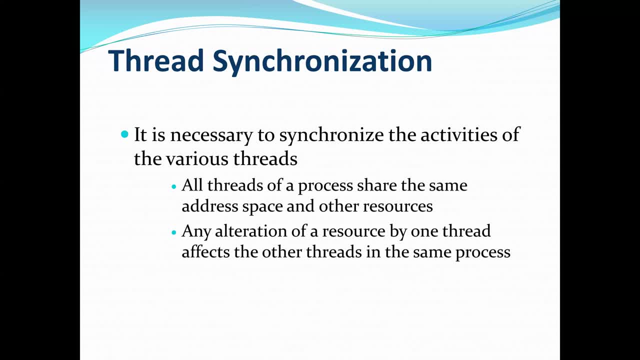 So, for example, if two threads try each try to add an element to a double linked list at the same time, one element may be lost Or the list may end up malformed. So the issue raised and the techniques used in the synchronization of threads are, in general. 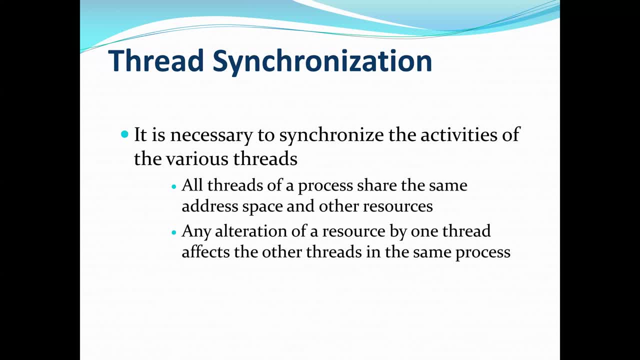 the same as for the synchronization of process, And again we will cover this concept in our textbook, again chapter five and six. So any alteration of a resource, resources, by one thread, We will surely affect the other threads in a same process. 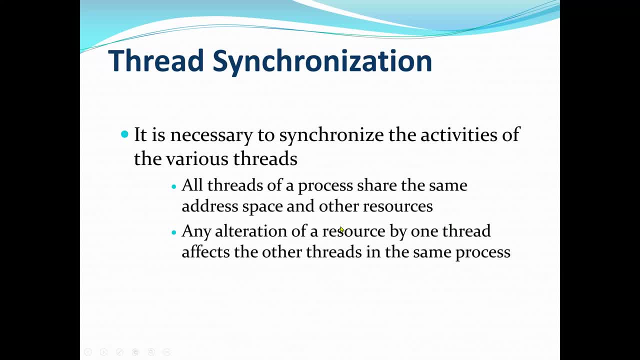 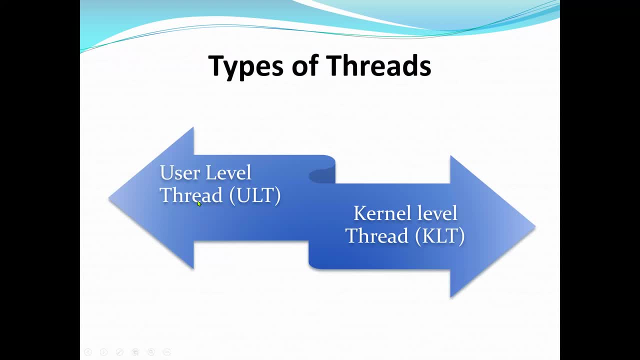 So this: why, again, we need thread synchronization. So we have two types of threads: The user level thread and also we have the bae-kene level thread. So again, they are two broad categories of thread implementation, either the user level or the kene level thread. 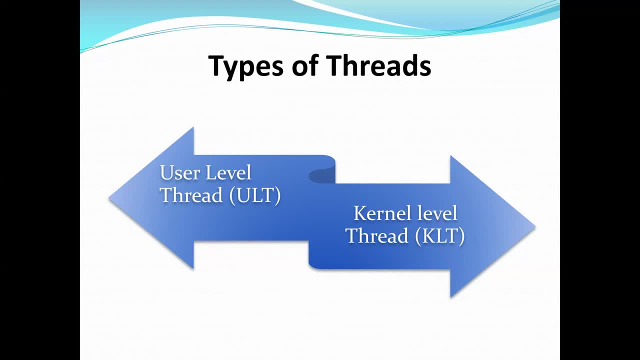 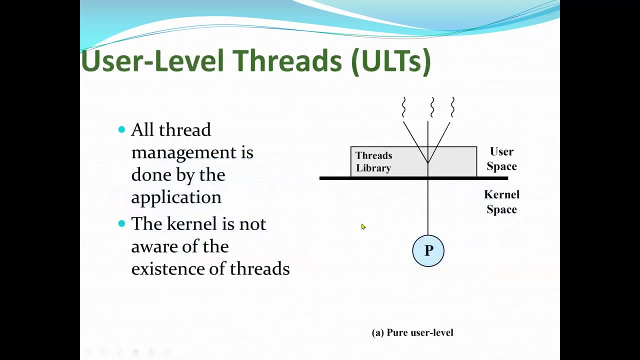 It's also referred to in the literature as the kernel support threads or lightweight process. That is the kernel level thread, So we shall go through each one. The first is a user level thread. So again, in a pure user level thread facility, all of the work of a thread management is done by the application and the kernel is not aware of the existence of threads. 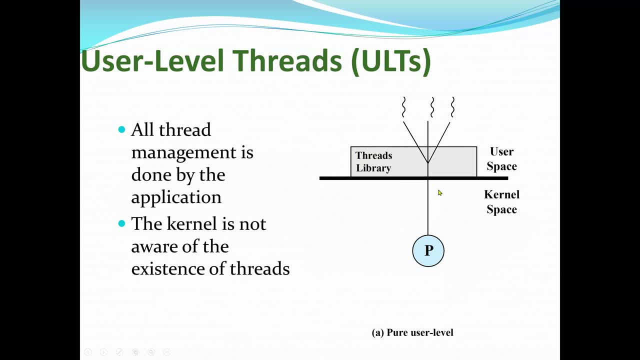 So this diagram can show, illustrate the pure URT, So the thread library files. we can see the user level at the top kernel level. down Again all the thread executing. they don't have any direct access or interfere with the kernel space. 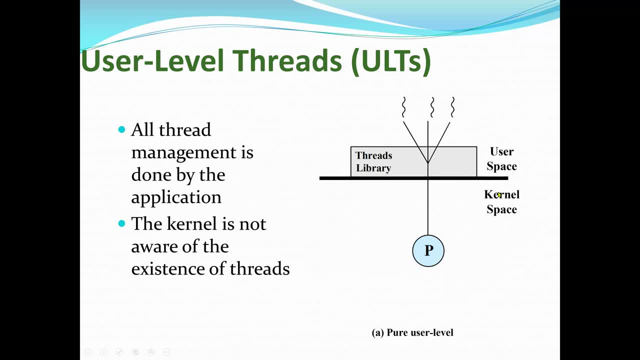 So sometimes we may call the user level thread as a very secure thread. So, again, all thread management is done by the application. The kernel is not aware Of the existence of those threads. So, again, any application can be programmed to be multi-threaded by using the thread libraries, which is again the package of a routine for user level thread management. 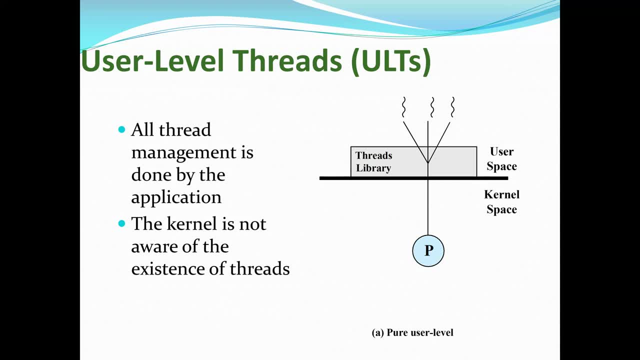 And this thread library contains code for creating and also destroying threads, Also for passing messages and data between threads, For scheduling thread execution And also for saving and restoring the thread contents. So again, by default an application begins with a single thread. 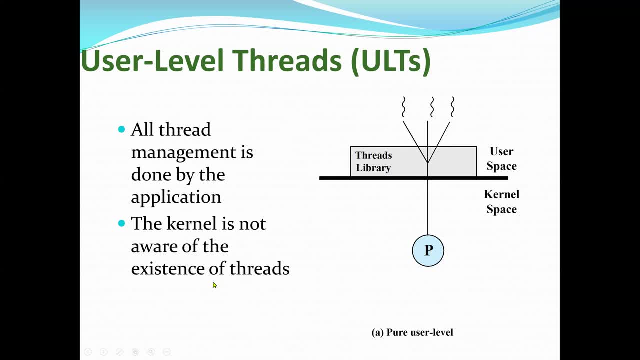 And also begins running in that thread. So if an application begins with a single thread and begins running in that thread, This application and its thread are allocated to a single process managed by the kernel. So at any time that the application is running, the process is in the running state also. 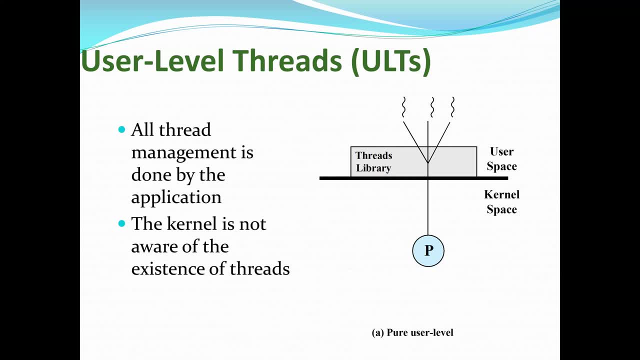 And the application may spawn a new thread to run within the same process. Spawning is done by invoking the spawn utility in the thread library. Also the control is passed to that utility by procedural call And also the thread libraries create a data structure for the new thread. 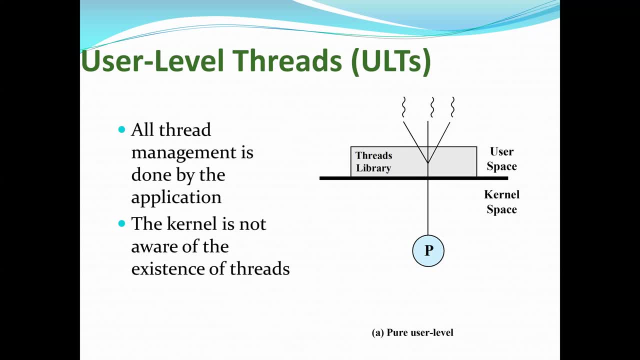 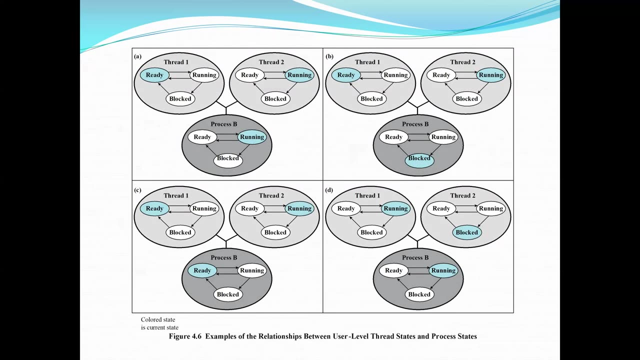 And then passes control to one of the threads within this process, And that process is in the ready state using some scheduling algorithm. So again, all of the activity described in the previous section- slides- again takes place in a user space And also within a single process. 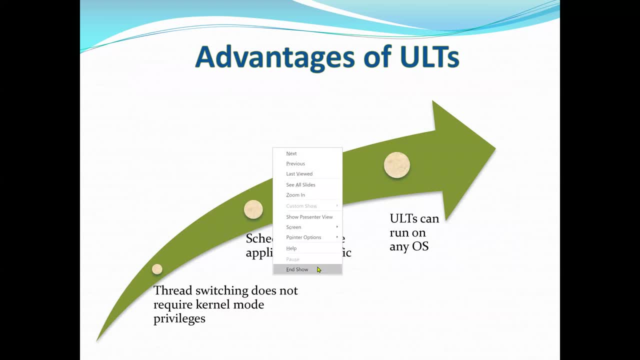 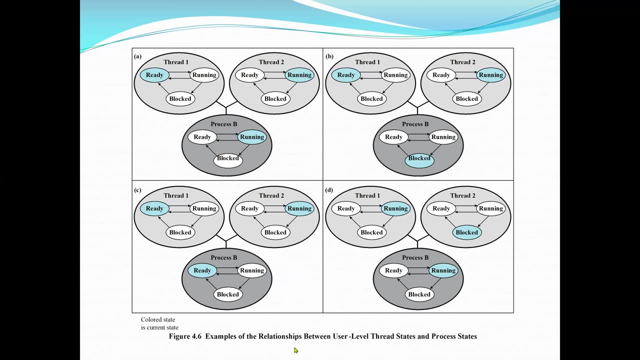 So again, this is So again. this is an example of a relationship between the user level thread state and also the process. So A. we have thread 1, 2. But both threads are in process B, So process B has two threads. 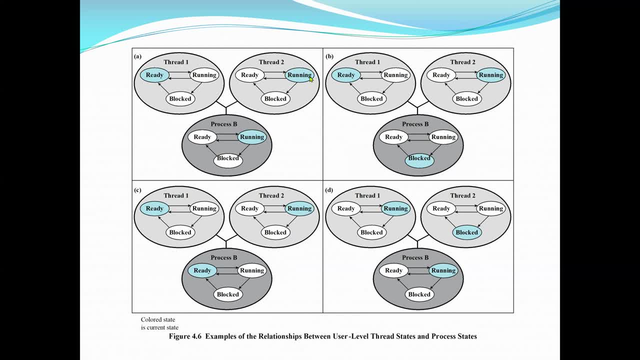 So we have to be in running state with the threads And now process B is in block But again our thread 1 is still ready, Thread 2 is running. Then when process B is in ready state, we have thread ready and running, etc. 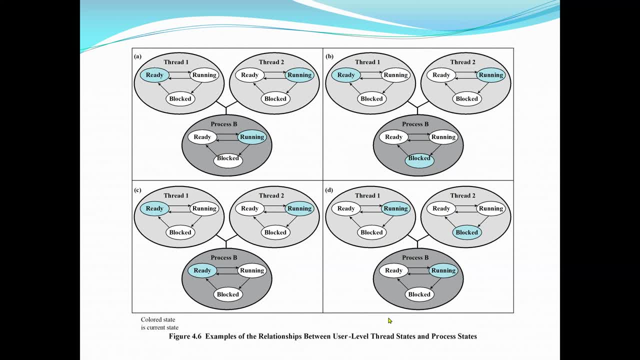 So the whole concept here is that the application executing thread 2 makes the system call that blocks B. So thread 2 make again block B. So again all of the activity described in the previous slides again take place in a user space and within a single process. 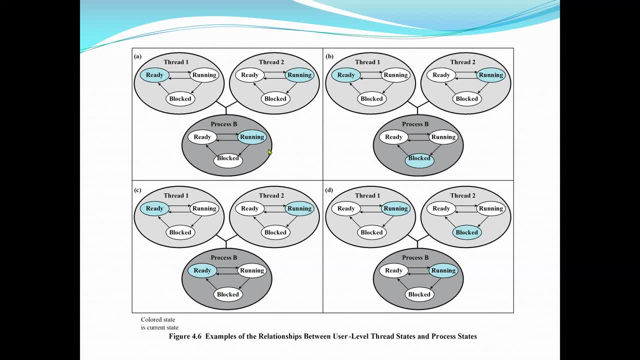 Now the kernel is unaware of this activity because this is a user level And also the kernel continues to schedule the process as a unit and assign a single execution state, Either ready, running, block, etc. To that process. So the example here again, number 1, we have application executing, thread 2 makes system call that blocks B. 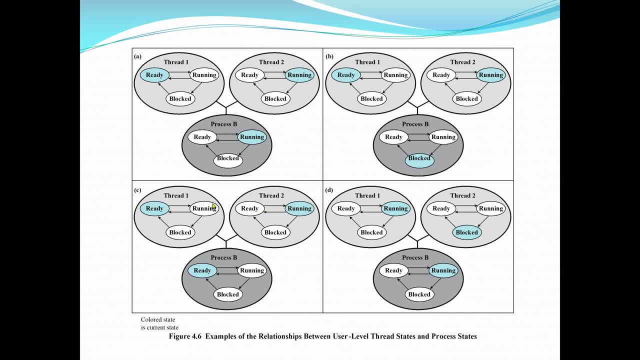 So, for example, an IO call is made And this causes control to transfer to the kernel And the kernel invokes the IO action, Then places process B in the block state And then switches to another process. Meanwhile, according to the data structure maintained by the thread library, thread 2 of process B is still in the running state. 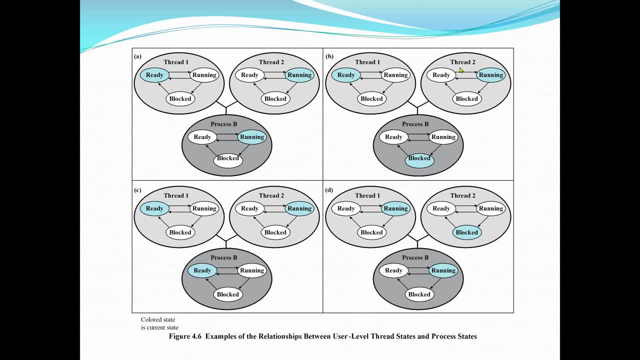 So this is important to note- that thread 2 is not actually running in the sense of being executed on the processor, But rather it is perceived As being in the running state by the thread library. So the corresponding state diagram are shown here in B. 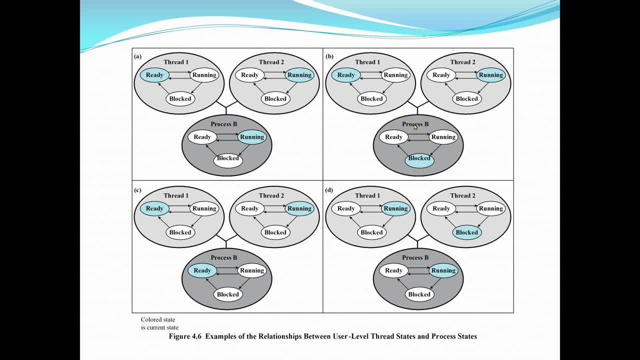 We can see, after some system call, process B was blocked. But we have: thread 1 is still ready, But thread 2 is in running state. Now let's say we have a clock interrupt passes control to the kernel And the kernel will determine that the current running process is in running state. 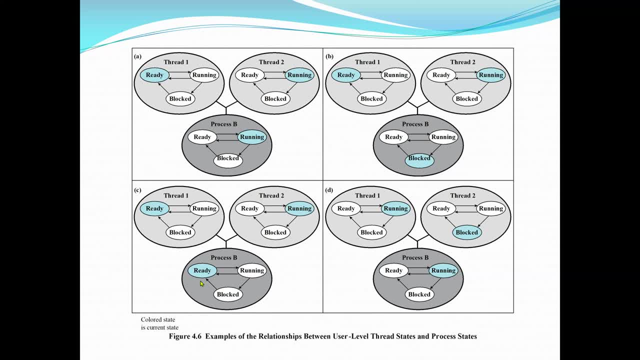 And the kernel will tell me that the current running process B has been exhausted its time. So the kernel now places process B again in ready state And switches to another process. But meanwhile, according to the data structure maintained in the thread library, thread 2 now of process B is still in the running state. 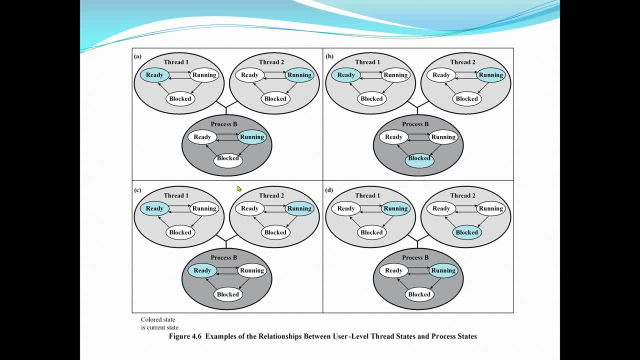 And the corresponding state diagram shows here. Now thread 2 is still in the running state. Now thread 2 has reached a point where it needs some action performed by the thread 1 of process B. So action must be performed by thread 1 of process B. 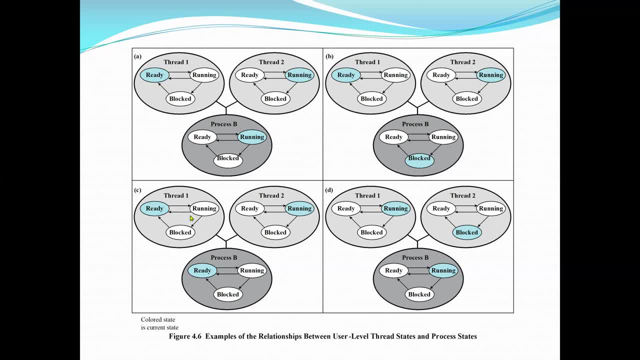 So thread 2 enters a blocked state And then thread 1 transition from ready to running state, Which is the transition from again ready to running. Now the process is to remain in the running state And the corresponding state diagram shows here again 4.6D. 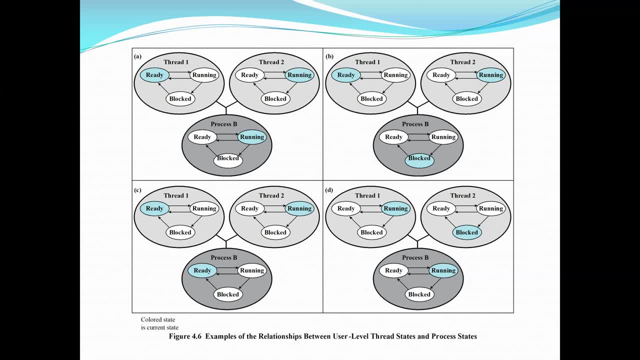 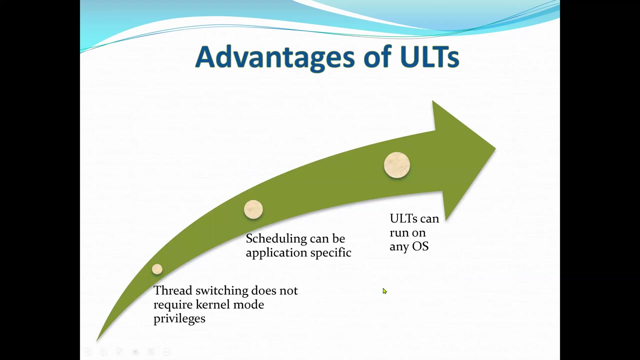 So we can note that each of the three preceding items suggest an alternative event, starting from diagram A all the way to B, C and D. So again, there are a number of advantages to the use of user-level thread instead of the kernel-level thread. 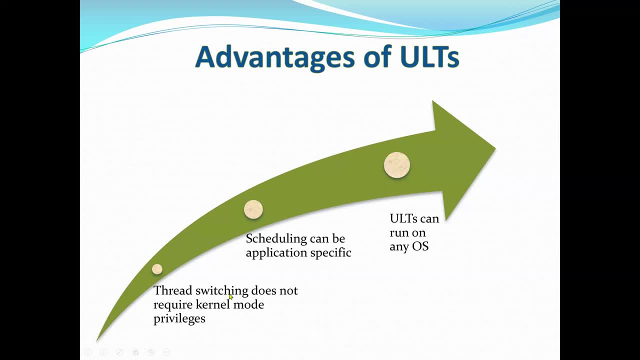 Including the following One: the thread switching does not require the kernel mode privileges. The thread switching does not require the kernel mode privileges. The thread management data structures are within the user address space of a single process. Therefore the process does not switch to the kernel mode to do the thread management. 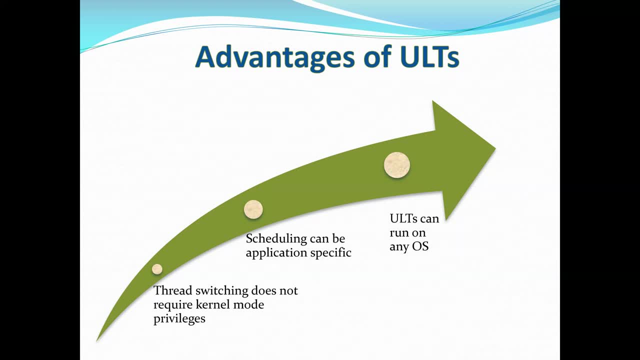 This saves the overhead of two mode switches, That's user to kernel or kernel back to user. Secondly, scheduling can be application specific. So that's an advantage. Scheduling, again, can be application specific. Now, one application may benefit most from a single or a simple run-robin scheduling algorithm. 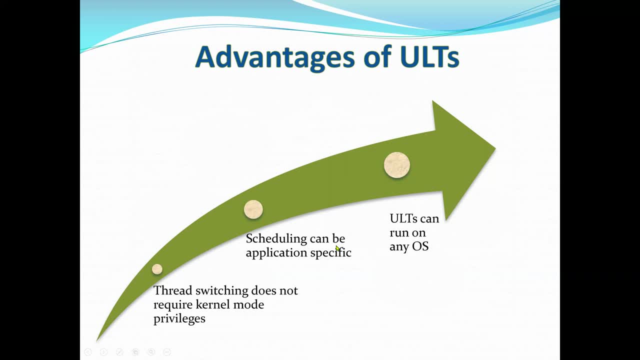 While another might benefit from priority-based scheduling algorithm. So the scheduling algorithm can be tailored to the application without disturbing the underlying operating system scheduler And also the user-level thread can run on any operating system And also the user-level thread can run on any operating system. 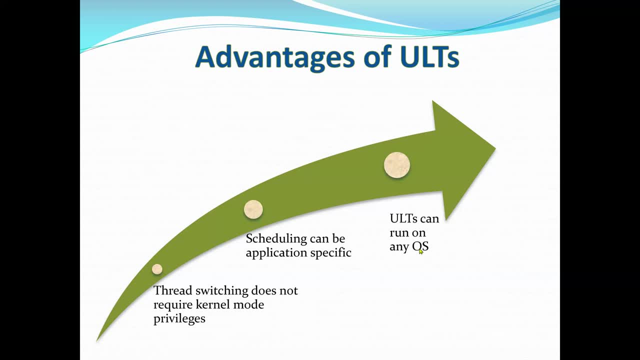 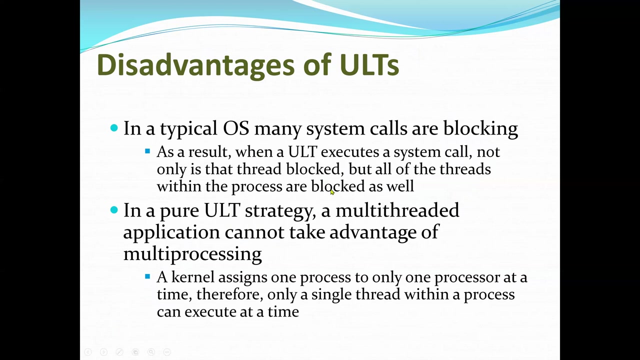 That's a good advantage. So no changes required. No changes required to the underlying kernel to support user-level threads. The thread library is a set of application-level functions shared by all applications. Now what are the disadvantages? Here we see again. there are two distinct disadvantages of ULTs. 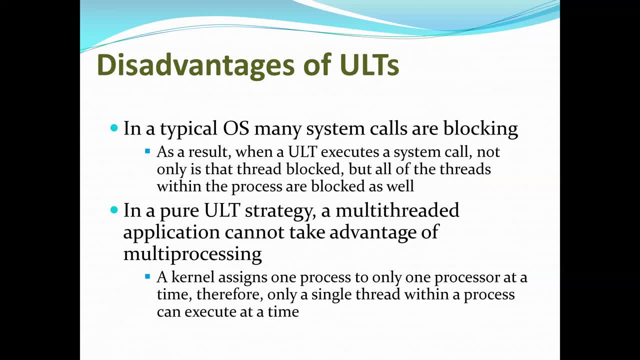 Comparing with KLT, There's a user-level thread comparing to the kernel-level thread. So in a typical operating system, many system calls are blocking. As a result, when a user-level thread executes a system call, not only is that thread blocked, but also all of the threads within the process are blocked, which we mentioned earlier. 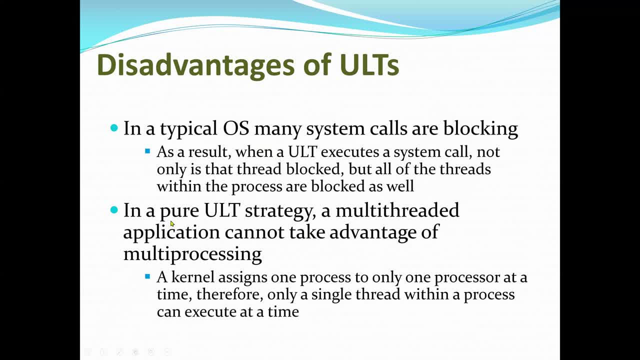 So that would be a disadvantage, And also secondly, in a pure ULT strategy. a multi-threading application cannot take advantage of multi-processing, So a kernel assigns one process to one processor at a time. Therefore only a single thread within a process can execute at a time. 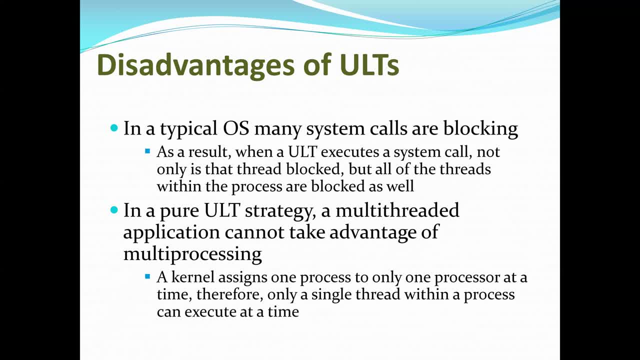 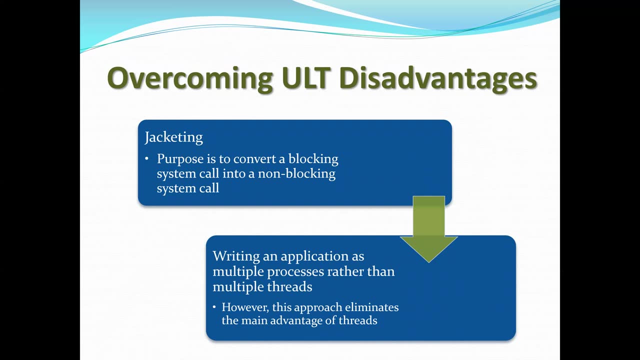 In effect we have application-level multi-programming Within a single process. Now overcoming the user-level thread disadvantage: Here we say we can use the method Jacketing. So another way to overcome the problem of blocking threads is to use a technique referred to as Jacketing. 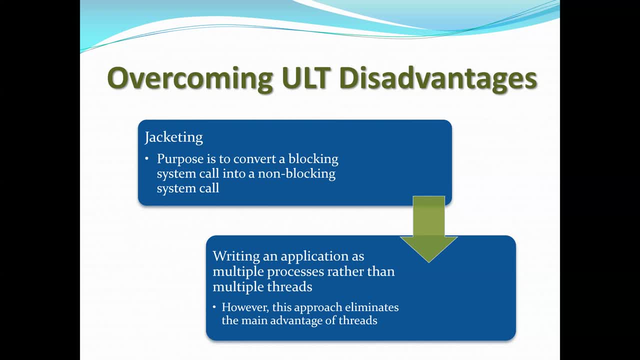 Now, the purpose of Jacketing is to convert a thread into a multi-threading application. The purpose is to convert a blocking system call into a non-blocking system call. So the purpose is to convert a blocking system call into a non-blocking system call. 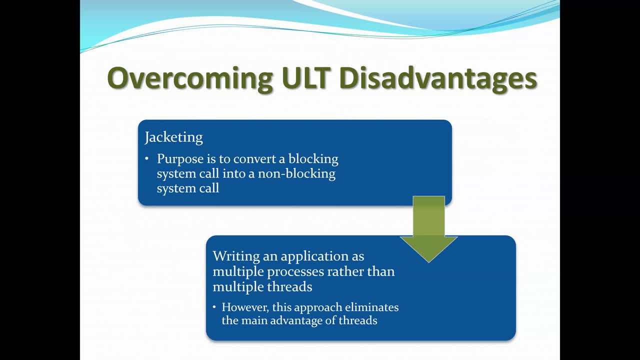 For example, instead of directly calling a system IO routine, a thread calls an application-level IO Jacket routine. Now, within this Jacket routine is code that checks to determine if the thread is blocked or not. Now this Jacket routine checks to determine if IO device is busy. 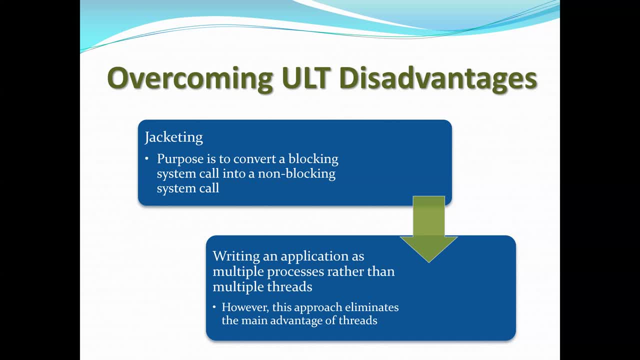 Now, if it is busy, the thread enters the blocked state and passes control through the thread library to another thread. So when this thread later is given control again, the Jacket routine checks the IO device again. So this is our kernel-level thread. 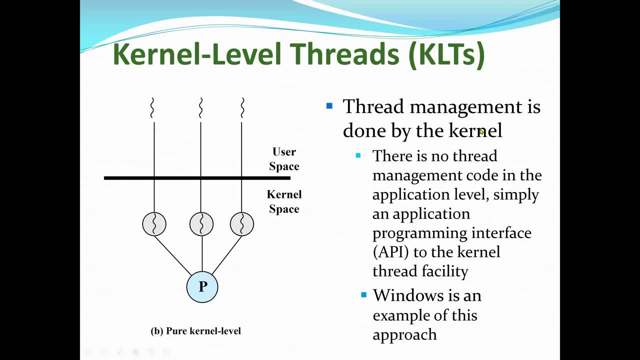 Again, this figure shows a block. This figure shows a thread management is done by the kernel with the kernel-level thread. So again, in a pure kernel-level thread facility, all of the work of thread management is done by the kernel. There is no thread management code in the application level. 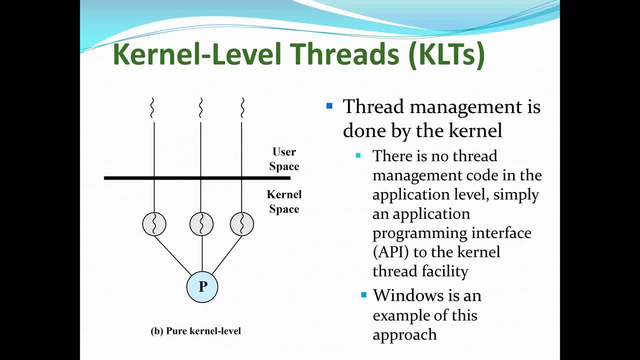 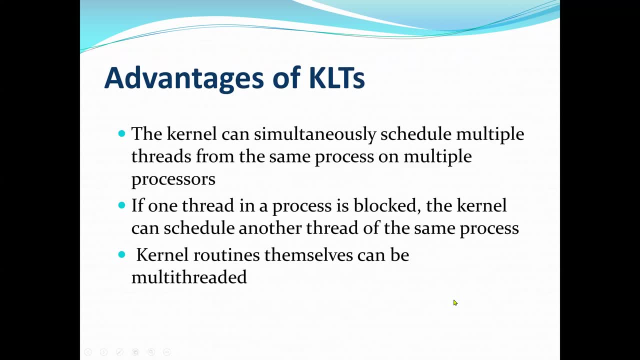 Simply an application program interface to the kernel thread facility. Windows is a very good example of this approach. Also, scheduling of a thread is done on a thread basis, Advantage of the kernel-level thread. a kernel can simultaneously schedule multiple threads from the same process on a multiple process. 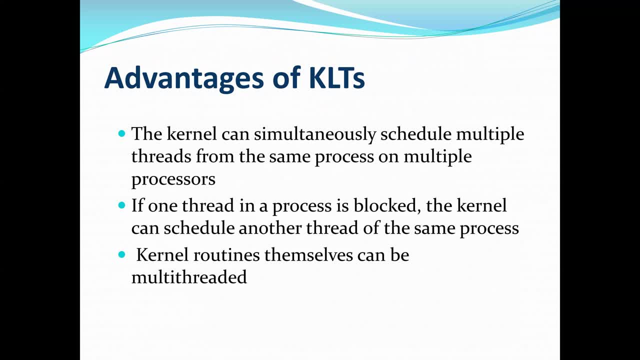 And also again, the schedule takes place in the thread basis. This approach also overcomes the two principal drawbacks of the user-level thread approach. First, the kernel level thread. First, the kernel can simultaneously schedule multiple threads from the same process on a multiple processes. 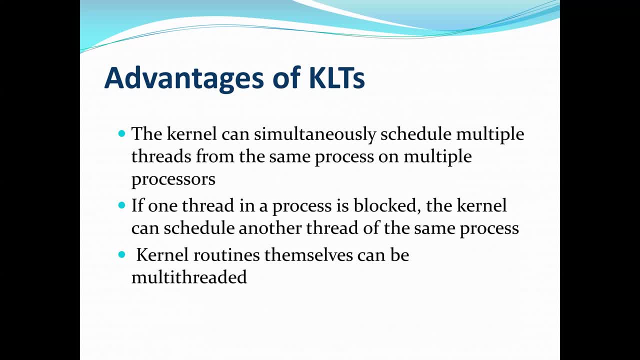 And second, if one thread in the process is blocked, the kernel can schedule another thread of the same process Again. another advantage of KLT approach is the kernel routine themselves can be multi-threaded. Again, the kernel routines themselves can be multi-threaded. 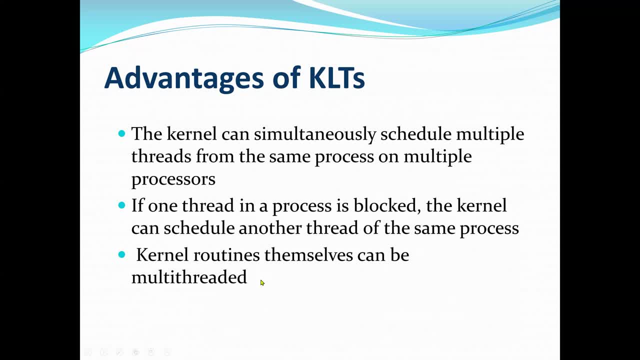 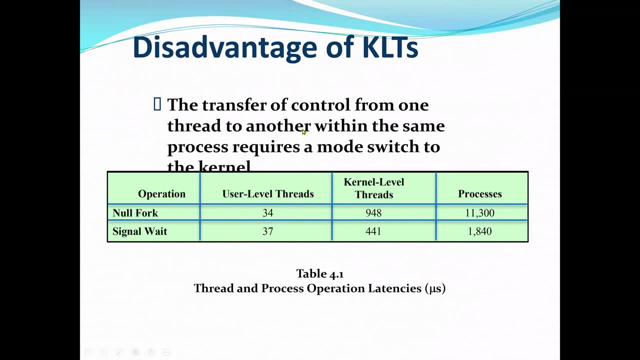 Again, the kernel routines themselves can be multi-threaded. Again, the kernel routines themselves can be multi-threaded. Now, the disadvantage of KLT here, we say, the transfer of control from one thread to another within the same process require a mode switch to the kernel. 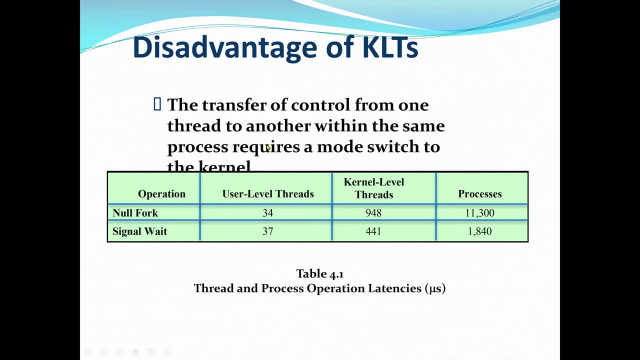 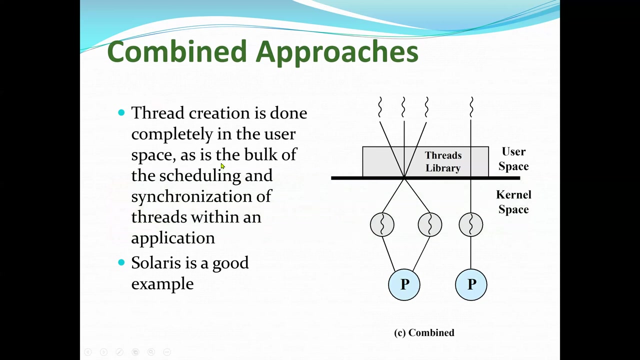 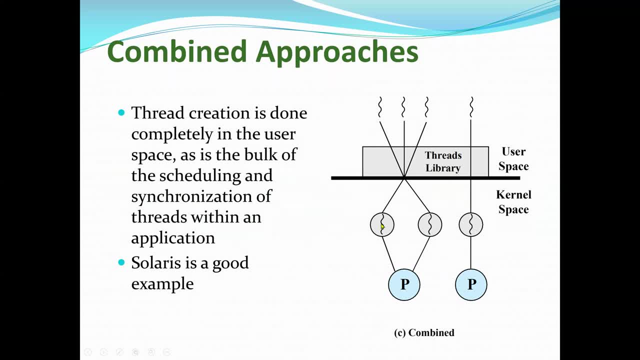 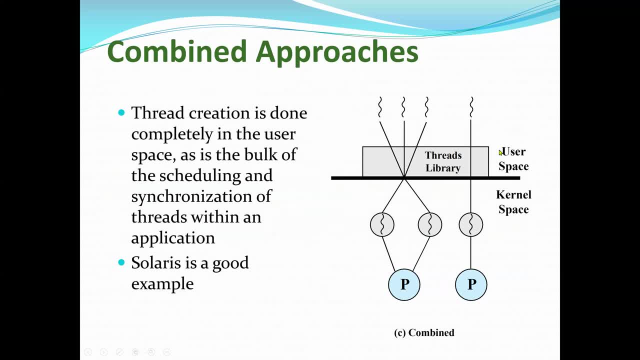 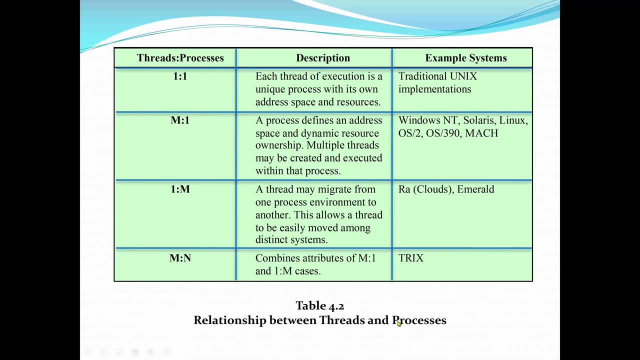 to ULT approach. comparing to ULT approach. comparing to ULT approach. comparing to ULT previous approaches. previous approaches, previous approaches stocks relationship between trace and also the process, so we may have one-to-one relationship, which means each trade of execution is a unique process within its own address, space and resources.